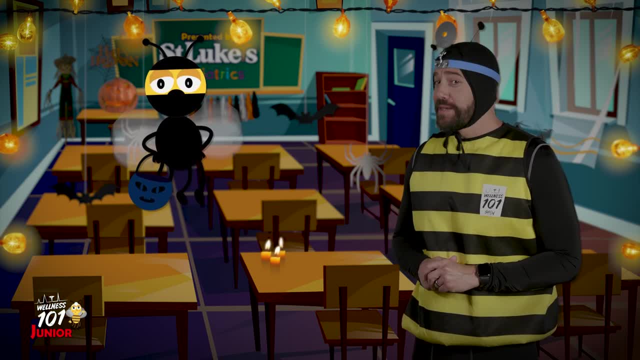 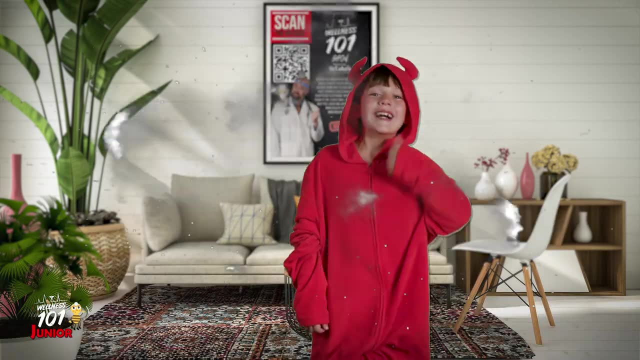 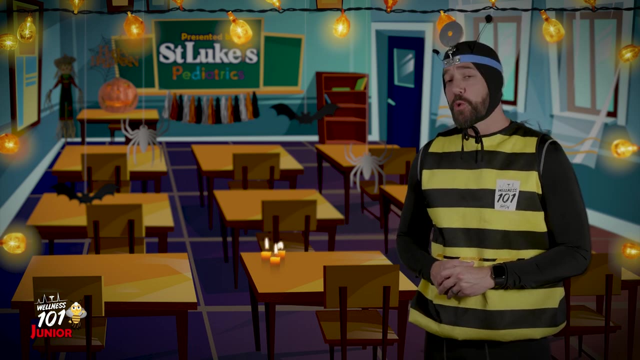 and the kiddos here should have a little chat about some Halloween safety tips. Step one: stand out. Halloween costumes come in all shapes, colors and sizes. It's fun to be a different character every year, but remember, gang, you'll most likely be trick-or-treating at 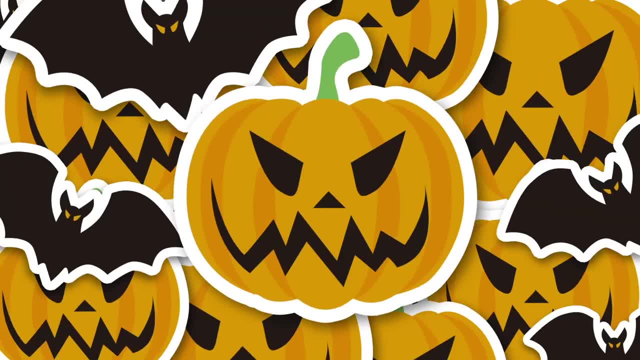 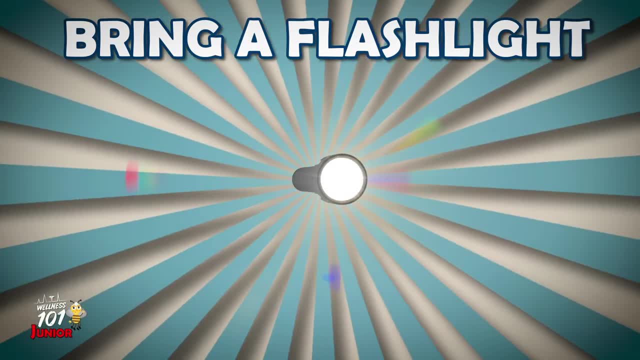 night. so it's a good idea to stand out in the dark. Try fastening some reflective tape to the front and back of your costume so that it stands out more than theерхandtheback of your costume, and to your trick-or-treat bag. It's also a good idea to bring along a flashlight or some glow. 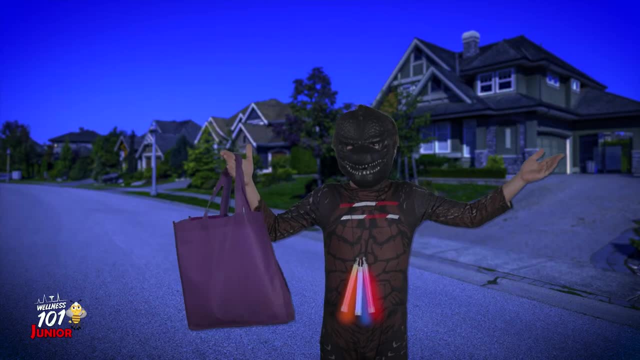 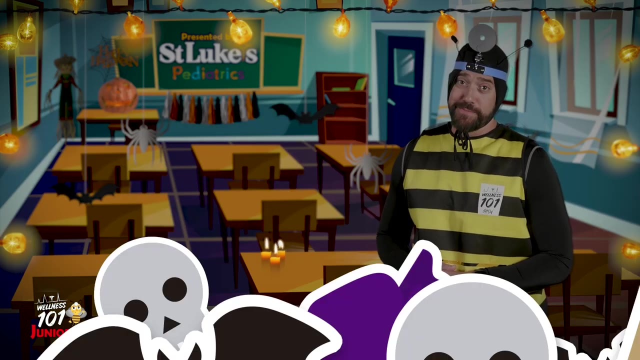 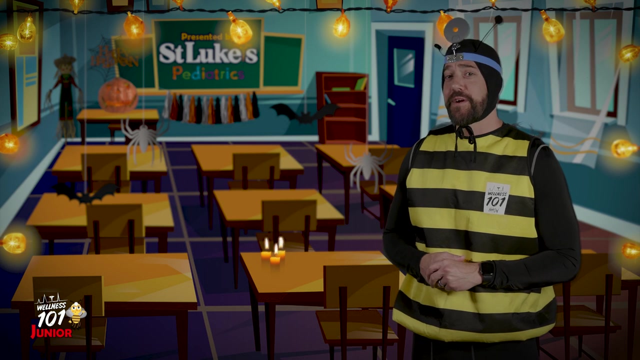 sticks that will not only help you see at night, but for others to see you. Step two, walk, don't run. The excitement of Halloween can be pretty overwhelming. It can be very easy to want to run from house to house to load up on all that candy. But this is a bad idea, my friends. Halloween. 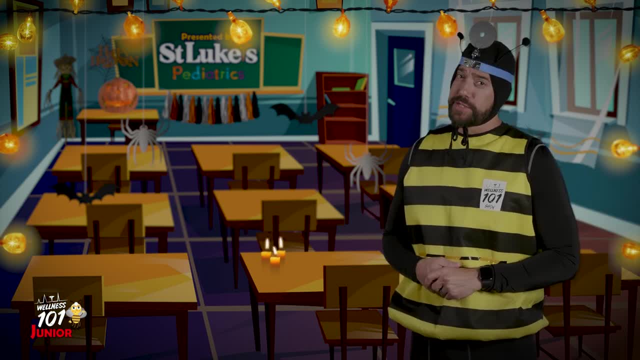 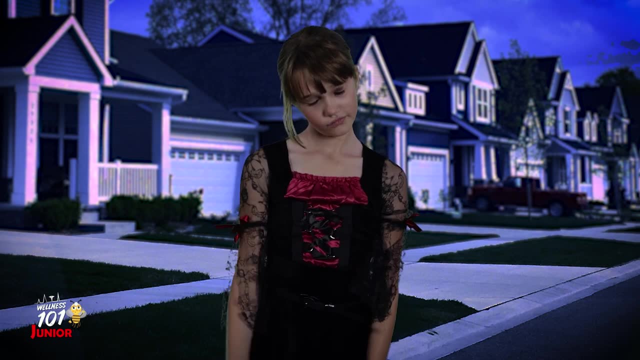 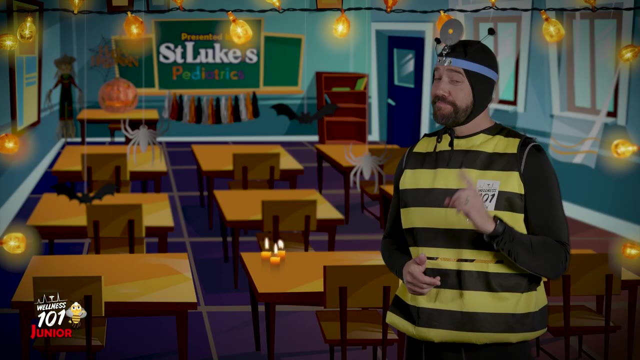 costumes can be bulky and usually come with all kinds of accessories, and you could easily injure yourself on these items. if you trip and stumble, Put your electronic devices down, keep your heads up and walk. don't run across the street. Trust me, gang, the candy will still be there, even if 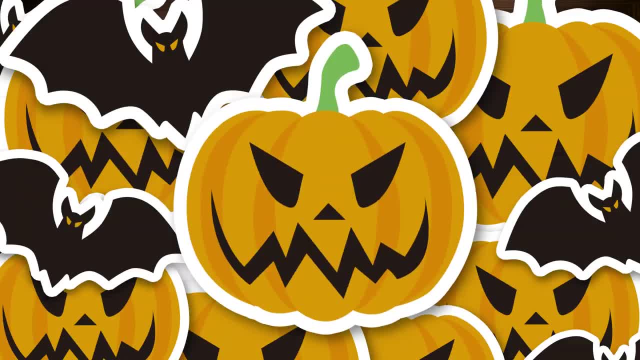 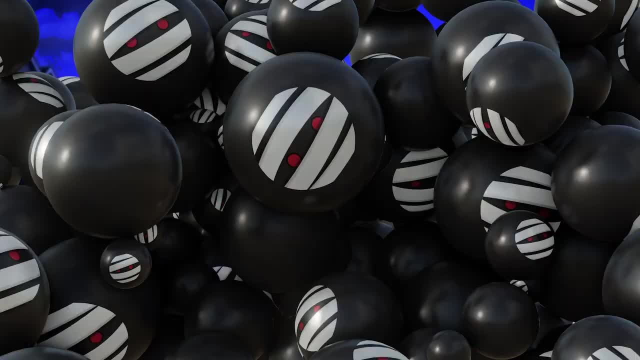 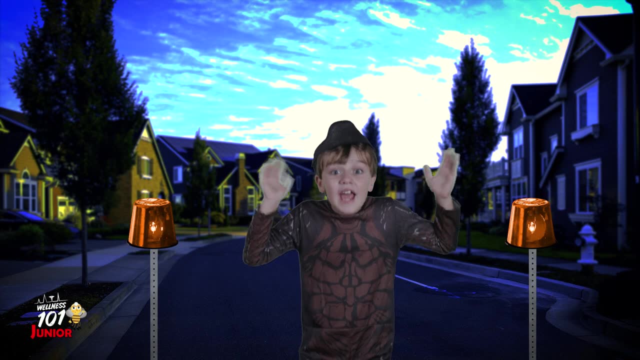 you walk. Step three: make eye contact. This tip goes way beyond Halloween. When crossing the street, never assume that drivers can see you. You want to make eye contact with them, to grab their attention. You may even try throwing them a little wave to make sure that they see you. 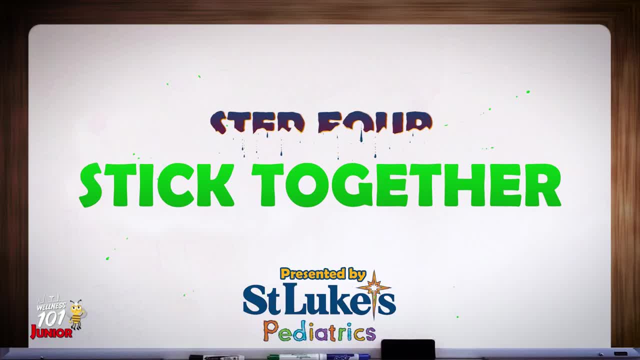 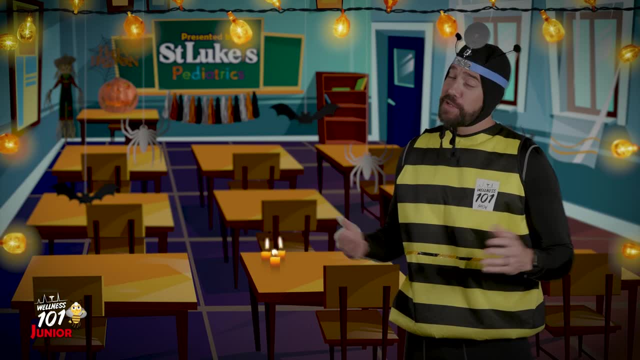 before you cross the street. Step four stick together. If you're under the age of 12, make sure you grab an adult to join you while you trick-or-treat. If you're old enough to trick-or-treat without supervision, make sure you stick to familiar areas that are well-lit and always. 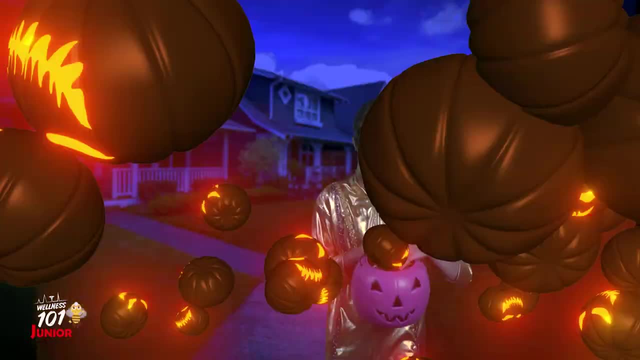 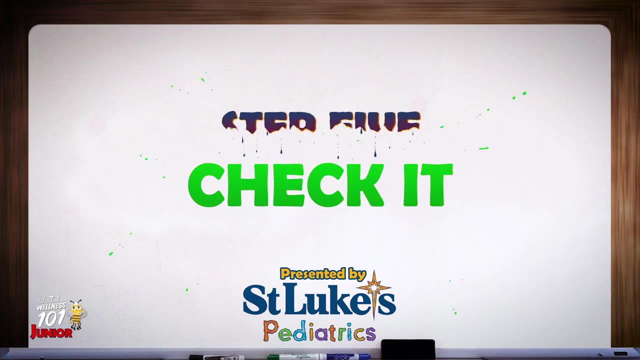 trick-or-treat in a group to maximize your Halloween fun. In this day and age, there are plenty of ghouls and goblins out there that would love to scoop up an innocent trick-or-treater. Step five: check it. Be sure, an adult checks. 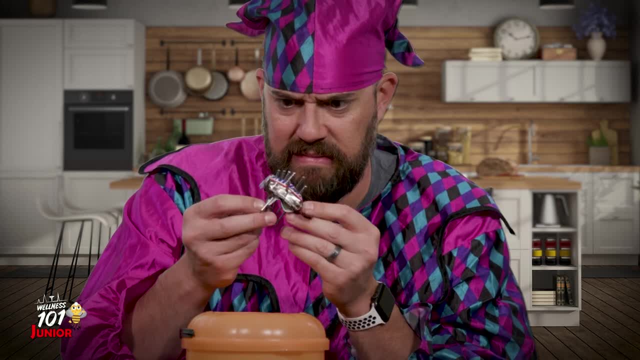 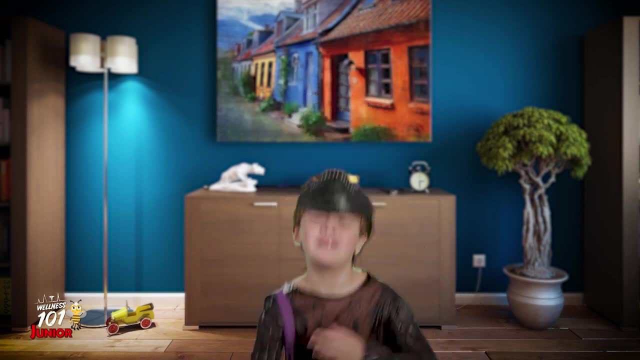 your candy haul for choking hazards and tosses away any candy that seems to have been tampered with. Lastly, don't forget to check yourself and limit the amount of treats you eat to avoid a stomachache. All right, my little ghosts and goblins question time. How do you stay safe?